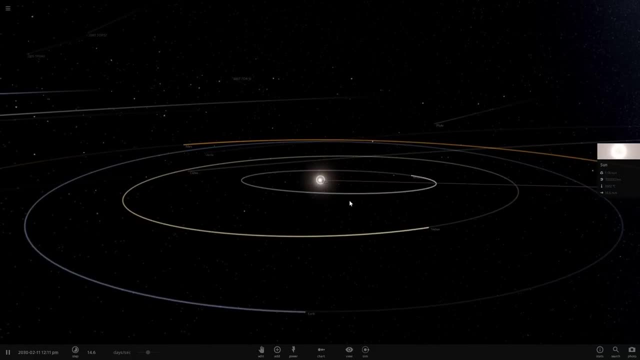 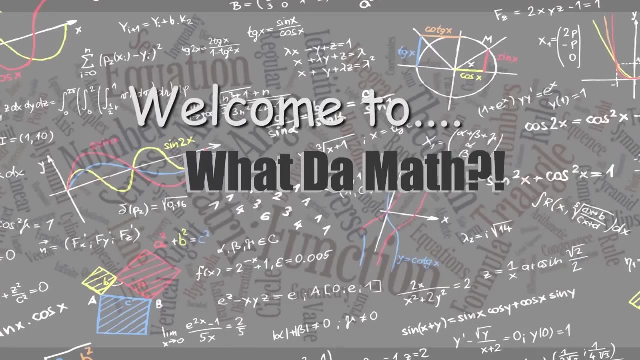 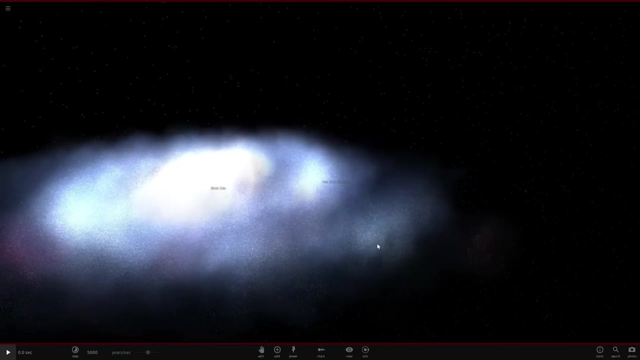 Sandbox 2 to try to recreate this early system, and I'm going to show you how it happens in the beginning. Welcome to What The Math. And so how does star formation start? Well, usually, not always, but usually it starts with a supernova. There's a supernova somewhere. 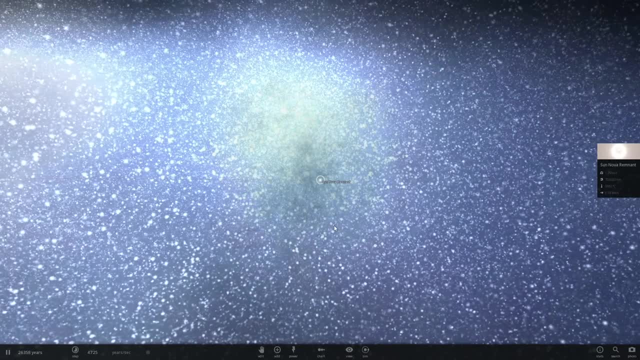 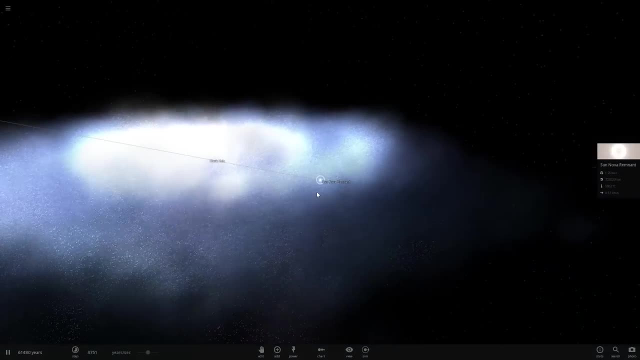 in the galaxy and it creates a very, very large cloud of gas, And so this gas starts to kind of move around in space and clump into little chunks. It doesn't always start with a supernova, because we've actually even found stars on the outskirts of our galaxy that were formed by 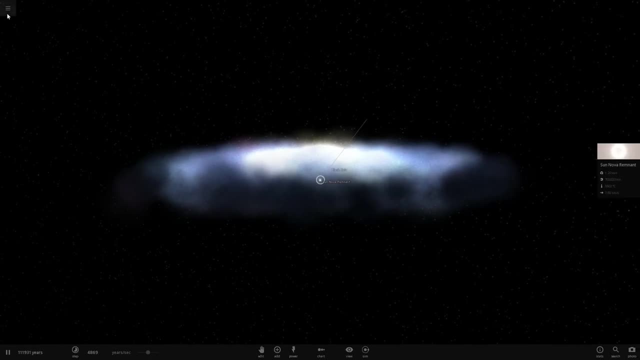 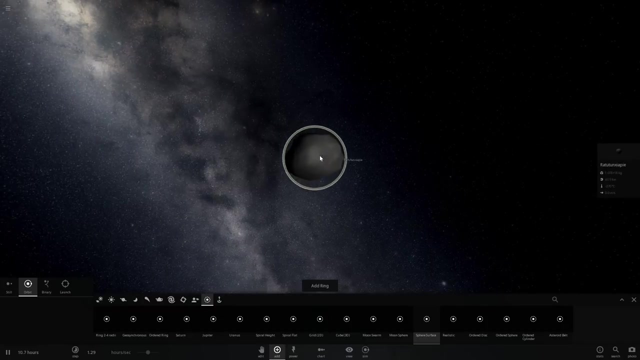 essentially, once again, material just clumping together. So once this actually starts, the gas in space starts to basically kind of move around and at some point one of the gas particles starts to kind of accrete into a slightly larger piece. Now this is a randomly generated asteroid. 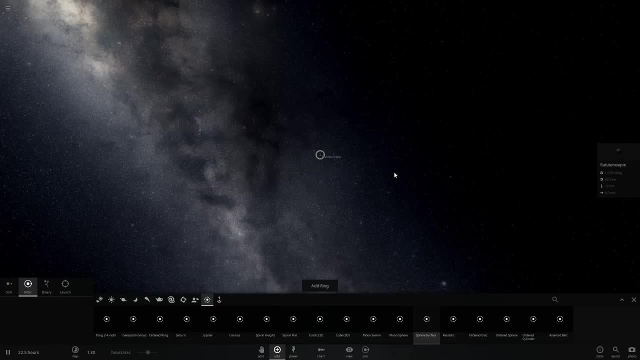 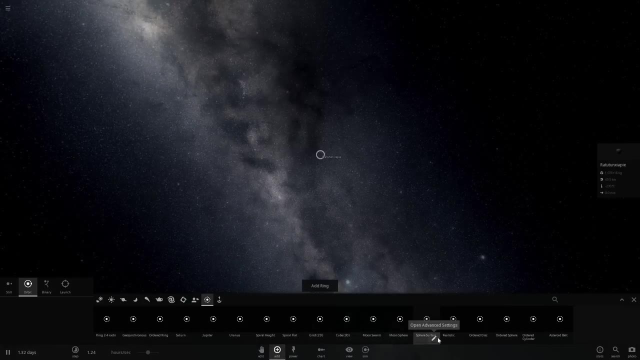 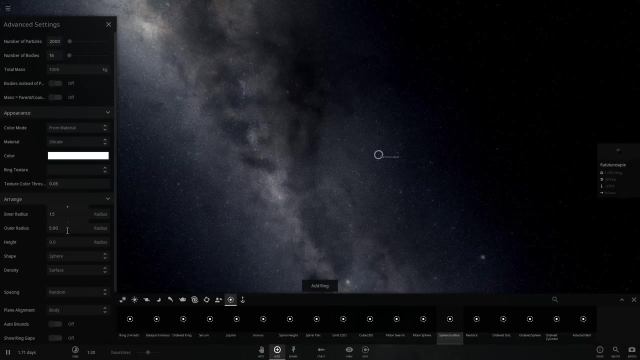 called Rototunxapi and that's what we're going to make into a star. So let's actually go into the add right here, add body, add rings, and we're going to add a sphere surface, just so you can visualize what this gas will look like. So we're going to make this from 1.5 to about 10 radii. 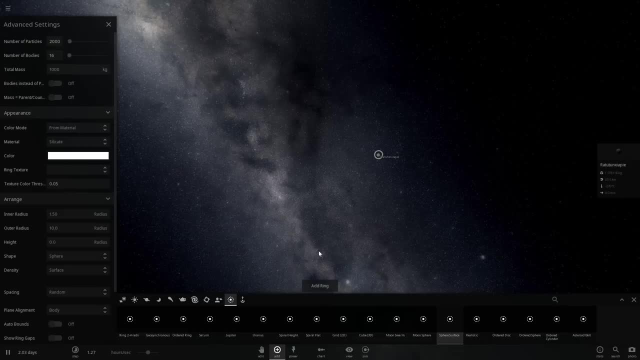 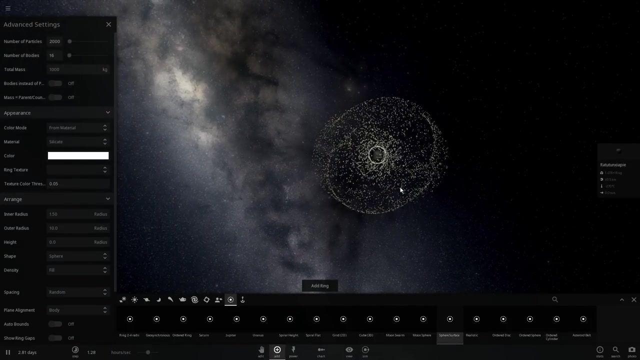 and let's actually start adding silicates at first. So here is what the actual surface will look like, but we're also going to do a fill here as well, just to have some inside stuff as well. So this gas starts to kind of orbit around a slightly larger piece and eventually it also 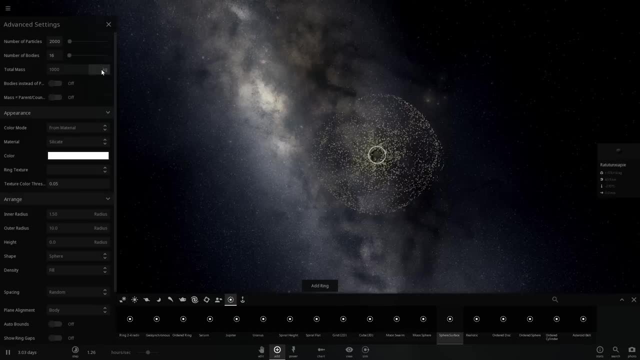 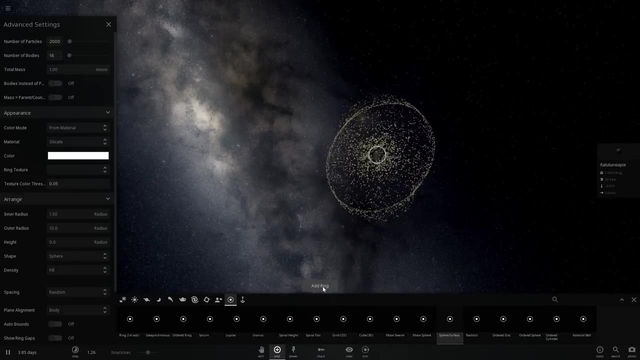 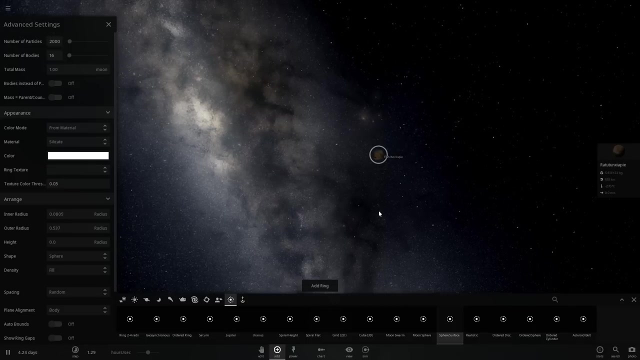 starts to coalesce on the inside. Now I'm going to start increasing the mass here. let's actually go into masses of moon and add maybe one mass of the moon to this object, and here we go. So instantly it became a relatively large piece. Now this is obviously a little bit accelerated. 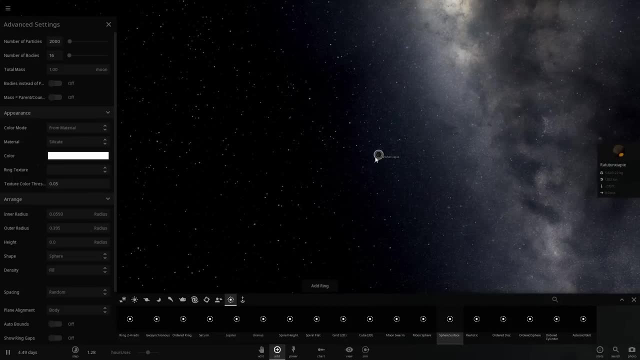 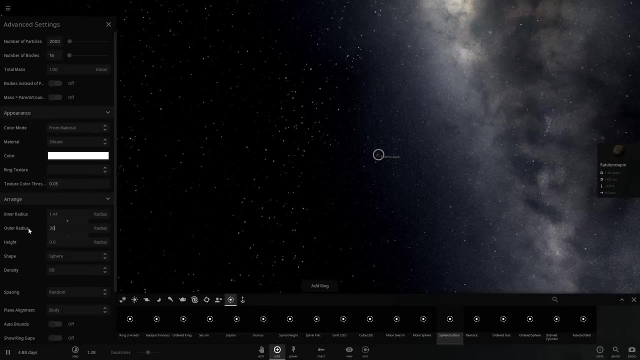 in terms of how it actually happens, because this will take thousands of years for it to coalesce into a large enough piece. but basically, as I keep adding more and more material, it will start growing growing inside. so there's our ring. it's sort of: this is obviously gas, it sort of orbits around. 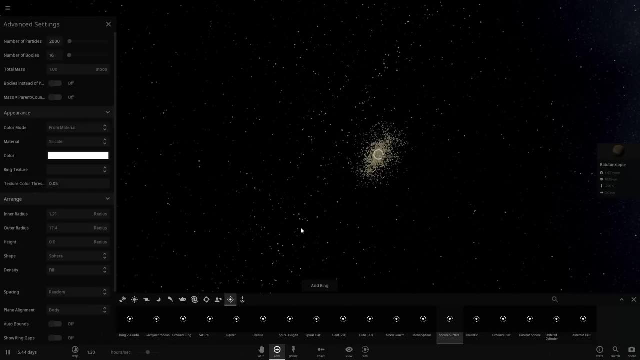 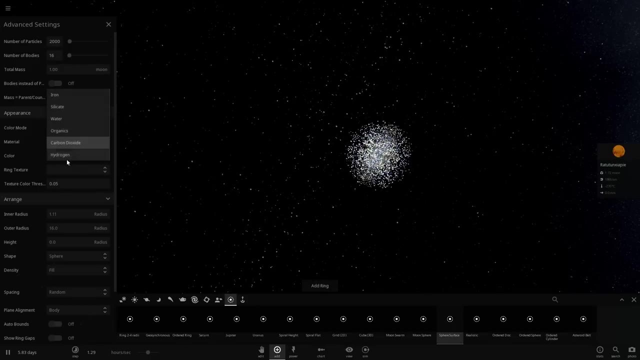 this little piece, and it's not just a ring, it's actually sphere of gas and there's going to be a lot of it and we're going to just add a bunch of other gas like water and carbon dioxide and, of course, hydrogen. now, most of it will be hydrogen, hydrogen and helium, and you can kind of see that. 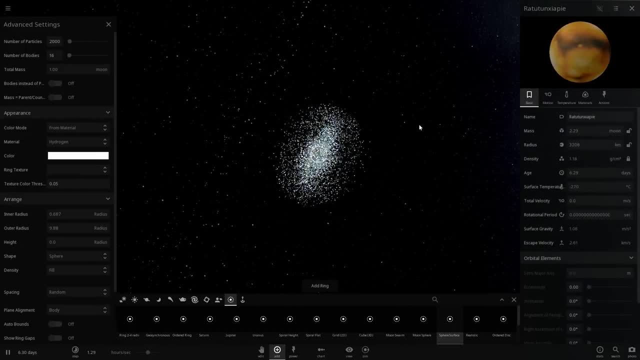 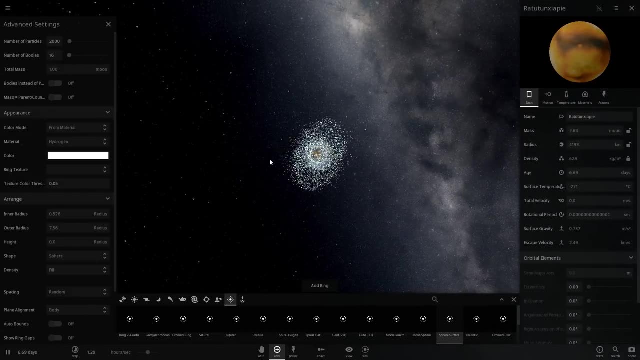 this object starts to basically receive a lot of these particles, a lot of them start falling into it, especially as it grows larger and larger in size. now this is a miniature model of this. obviously, this would be like everywhere this, the gas, will be everywhere. but as this object grows, 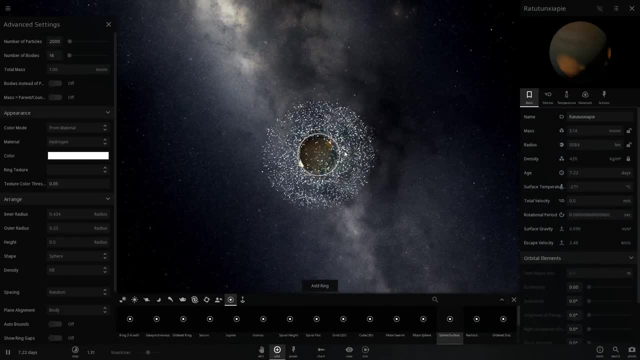 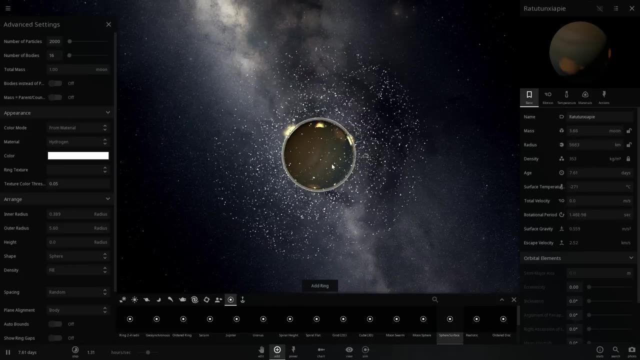 larger, the gas obviously gets to be attracted to this object and fall into it. so a lot of different explosions going on there and that's because this is this- is slowly growing. it's already you can kind of see the mass growing here. it's already at four masses of the moon. 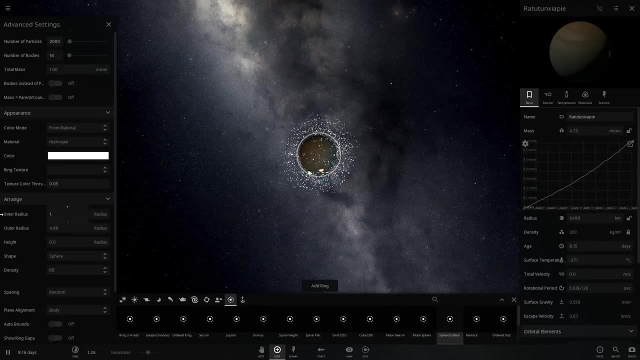 and getting larger and larger. so let's start adding a little bit more material here, a little bit more spheres, and possibly the mass here will be now 100 moons. let's just do it this way. so here we go, and i'm only going to be using hydrogen for now. 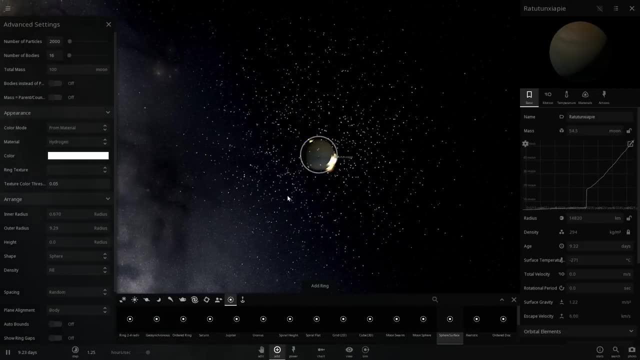 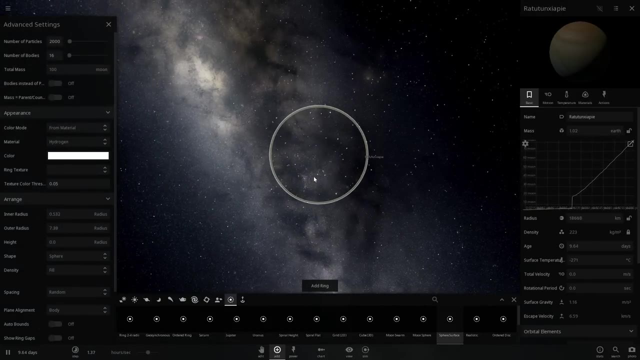 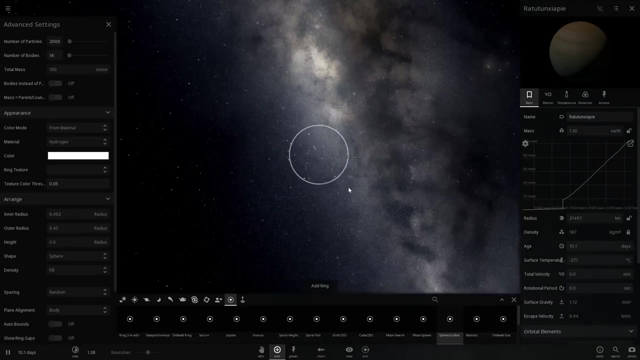 because most of the material here will very likely to be hydrogen or helium, and so this growth will be quite fast. and unfortunately, in this game sometimes this actually happens. if you, if your object, starts growing too fast, it sometimes disappears. now this happened to me before and was not able to solve this, unfortunately, so i may have to actually start this from scratch, but if 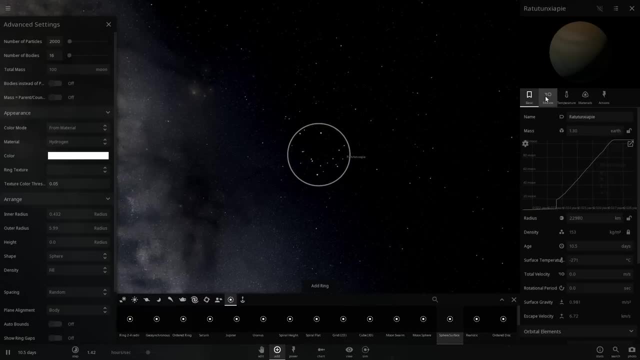 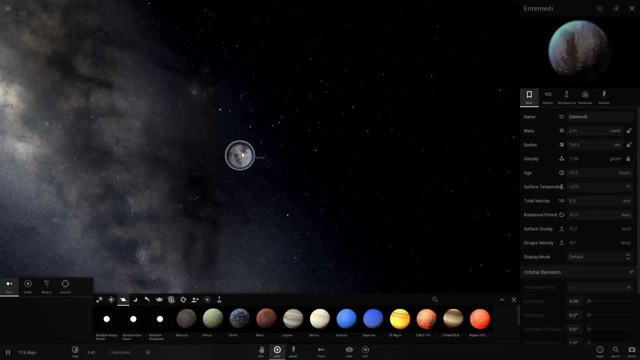 this happens to you, unfortunately you can't really do anything, but anyway. so let's just remember what the mass of this object was and also save the name, and unfortunately the name didn't really get saved, but anyway. so let's just start from here. so imagine this: is that that object that we had? 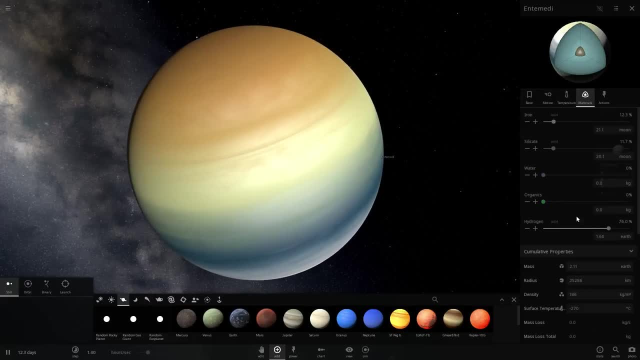 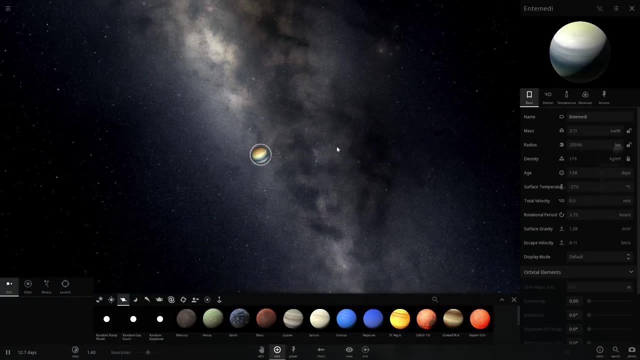 before. most of it was, of course, hydrogen, and so here we go. so this is a new object, basically still the same star. um, it's called antimediae. now, it's still actually not a star at all. it's still not a. this, as a matter of fact, it cannot be even called a star. it is not even a protostar, just yet. 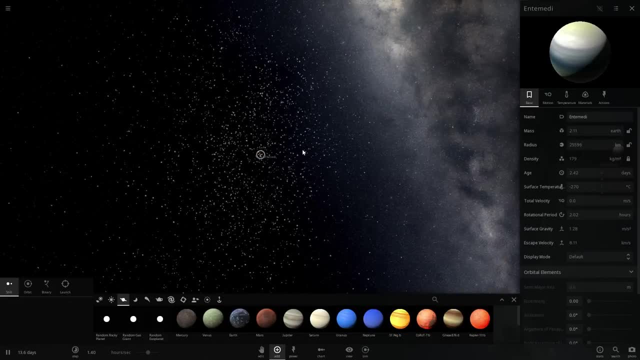 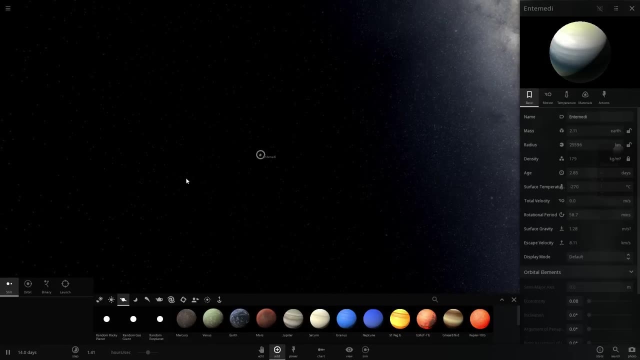 this is still a kind of a protostar like cloud, and there's going to be quite a lot of them after the supernova. as a matter of fact, there's going to be one here, there's possibly going to be one over there, there's going to be one over there somewhere. there's going to be quite a lot of them. 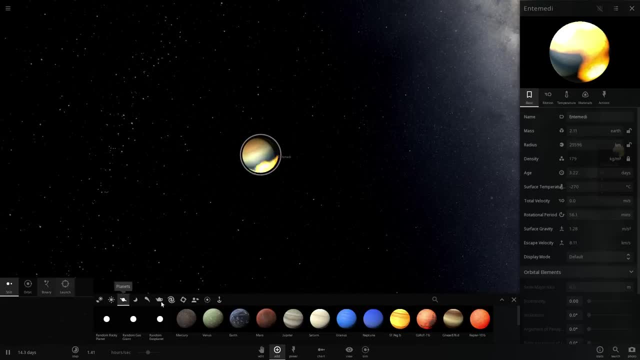 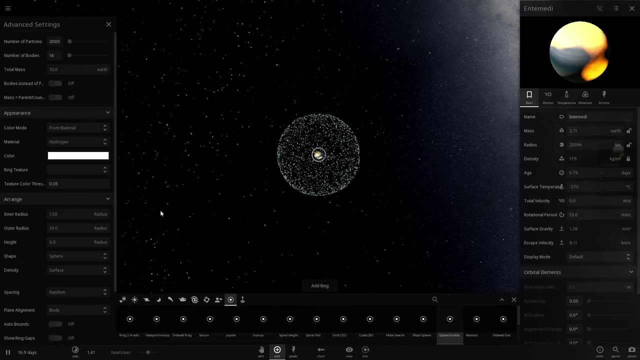 because this is how many of the stars usually are formed after the supernova event. but obviously there's going to be quite a lot of guests in this particular location as well. so we're going to recreate this again by adding more and more and more of these stars, and we're going to do that. 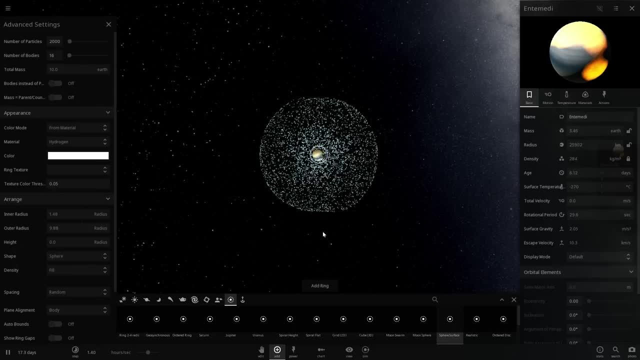 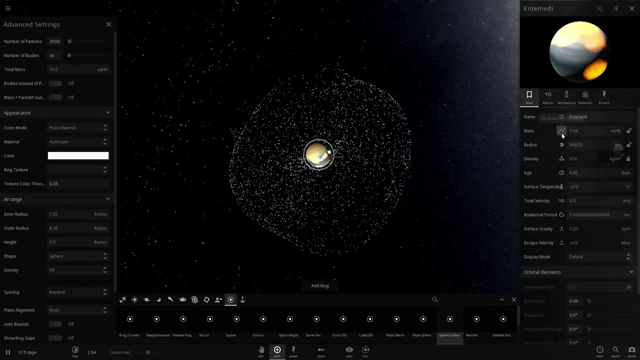 by adding more and more of these stars, and we're going to do that by adding more and more of these stars of gas, both in surface and fill mode, and so this will eventually start growing larger and larger and larger and obviously- and you can kind of see the mass increasing here- obviously as it acquires, 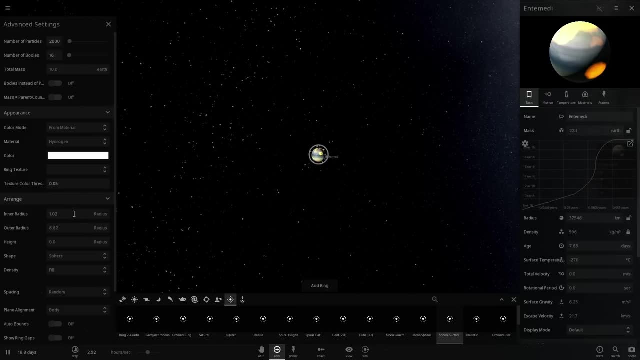 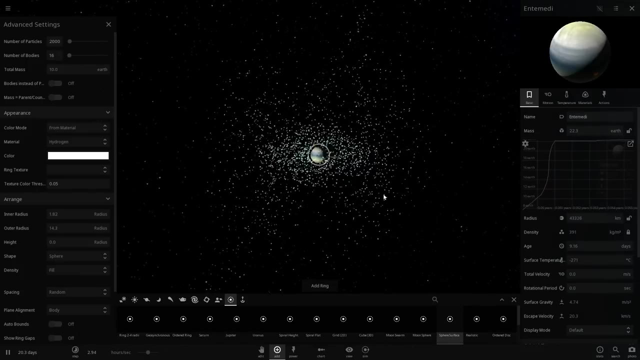 mass. it's going to approach closer and closer to that mass that it needs to become an actual, a legit protostar, and so what we're observing right now is actually called gas clumping. so basically, gas clumps into the center and is creating this um. 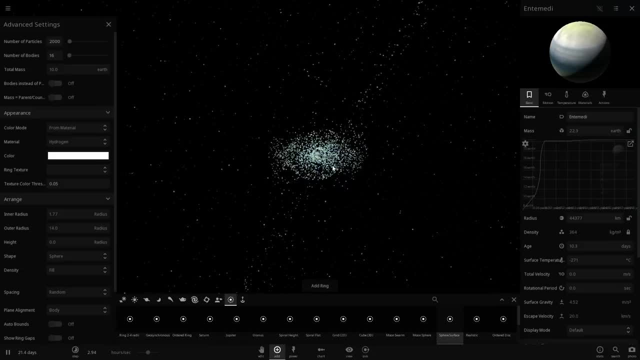 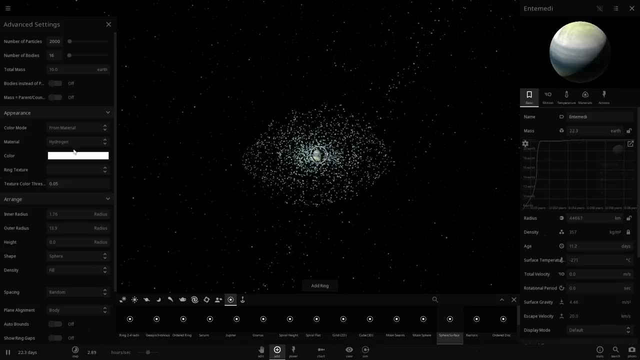 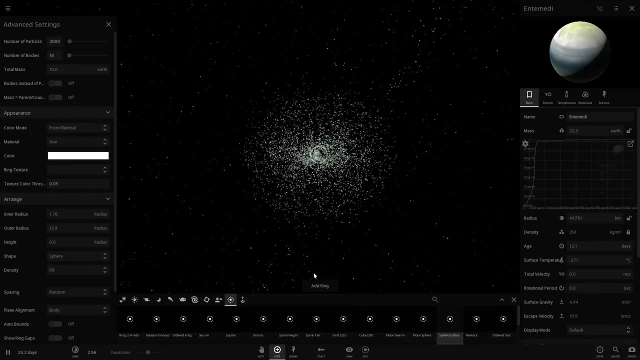 um, kind of a central region that usually grows pretty fast and becomes really really hot really fast as well. and so here, as i keep adding more and more of material, and let's actually just maybe add some just a little bit of silicates as well, just a little bit of iron, as we add more and more of 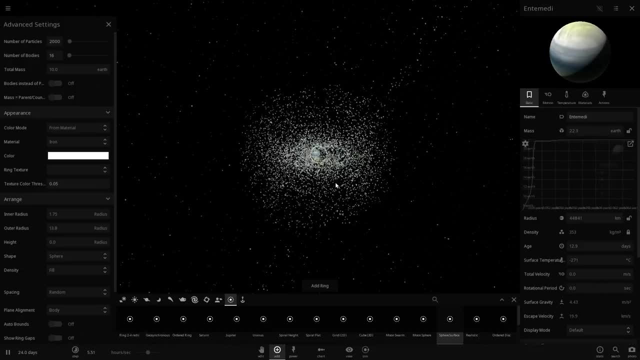 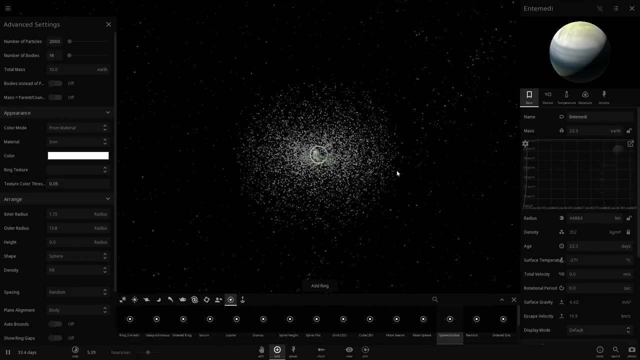 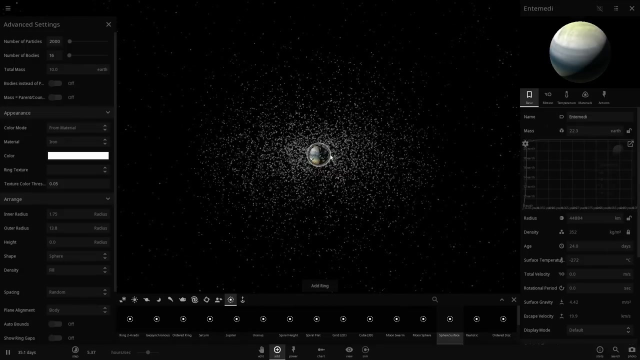 this stuff, it will obviously create a larger and more hot object and, as a matter of fact, as this becomes more clumped, the actual uh collapsing, uh starts to accelerate as well. so as this clump becomes more and more dense, it actually becomes almost transparent. so, um, the infrared radiation, the heat that escapes from here, actually, 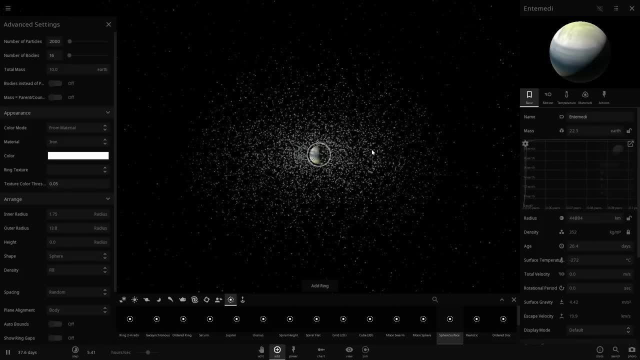 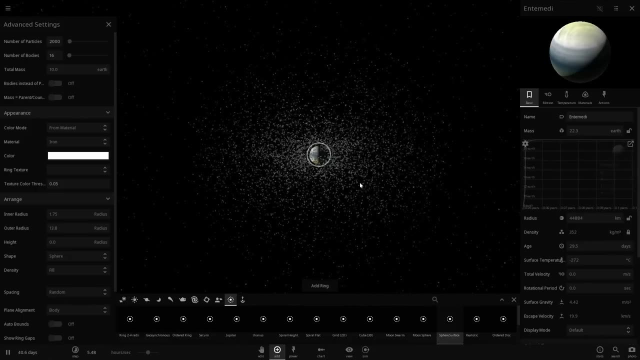 becomes trapped in um in the in this gas, and the pressure and the temperature on the inside starts to dramatically increase and at some point the pressure actually becomes so high that it prevents the uh inflow of more gas. as a matter of fact, it sort of develops like an outer shell, where it's 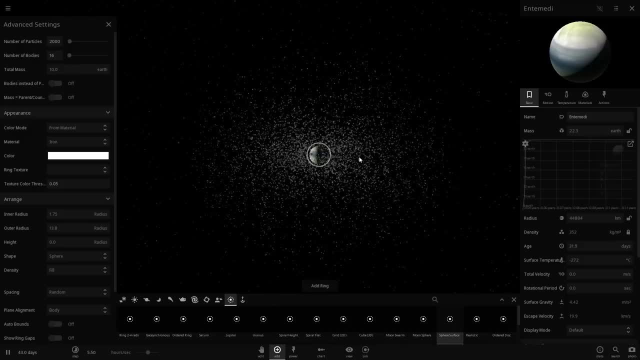 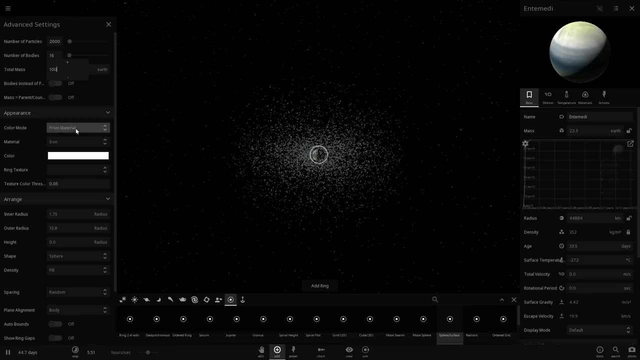 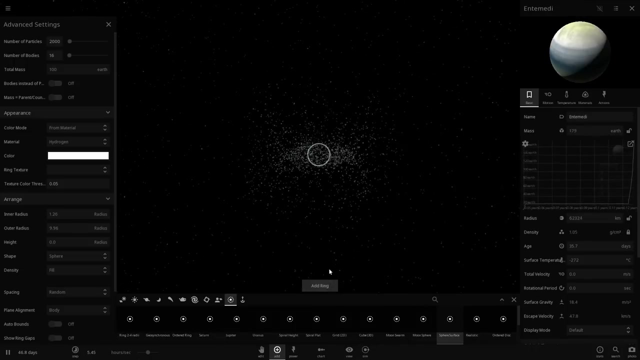 where no more gas is allowed to go inside, and this is what we would actually call a stable protostar. but we're not there just yet. we still need to add quite a lot more mass. so let's just keep doing this. let's add a little bit more hydrogen and increase the mass even more, and so here we go. this will. 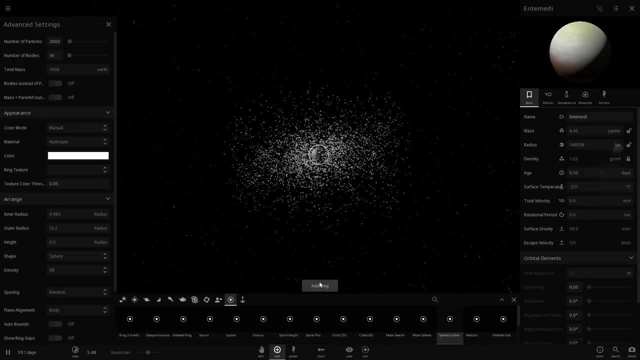 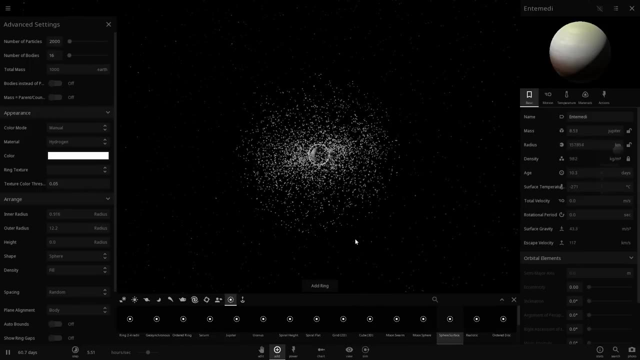 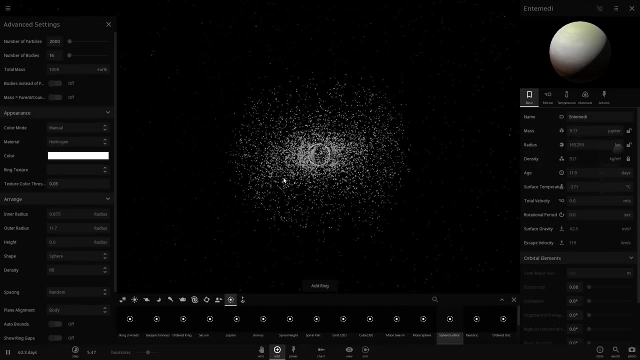 now start becoming more and more massive, and at first, when this protostar just kind of starts being created, it only really has about one percent of its final mass, so here it would be only about a few masses of drip um. but as it continues to grow, um, all of the material that is orbiting around it will eventually fall into it because obviously the mass becomes larger and attracts more and more material that orbits around it. and after a few million years of this, this is when we'll start seeing the nuclear reaction on inside. on the inside, because the hydrogen will actually reach temperature and pressure needed for it to start fusing um and creating quite a lot of energy. but we're not. 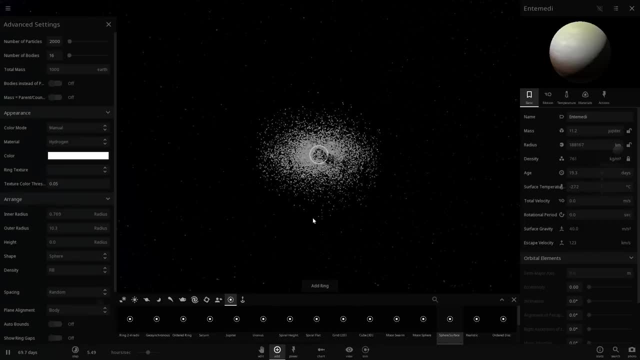 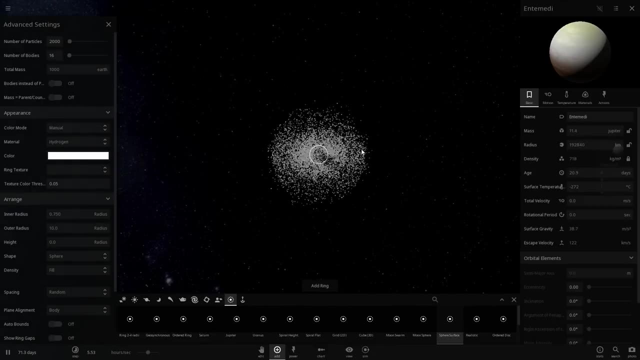 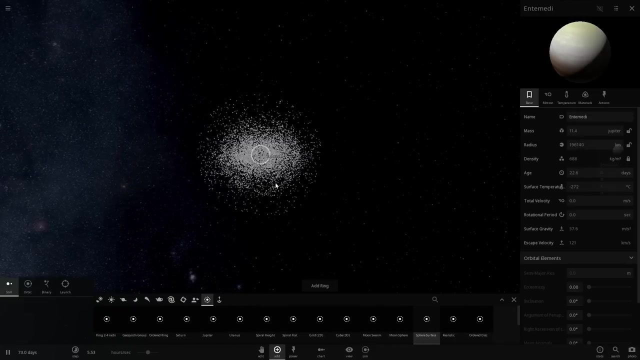 there just yet, because we still haven't reached that um, that particular period. we're still sort of in the period where there's a lot of sort of turbulence here, a lot of wind and most of the material from from this direction will actually be attracted to um, to the star, whereas um right here on top and on the bottom, because of the way that this star 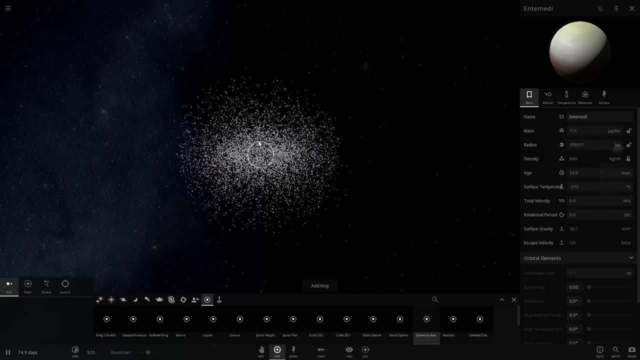 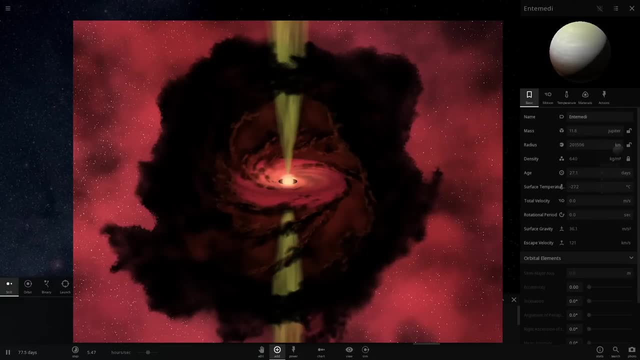 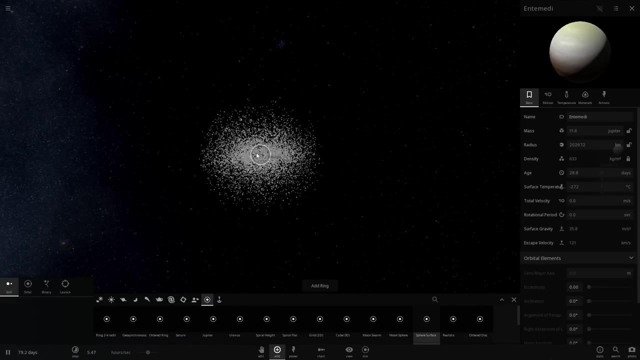 various sort of gases and with various sort of gases and with various sort of gases and with materials being thrown out completely, and these two jets will actually be with this star for several million years, until it actually becomes a main sequence star, when it really starts burning um hydrogen, and when all of this gas kind of disappears. but uh, just for now, let's actually 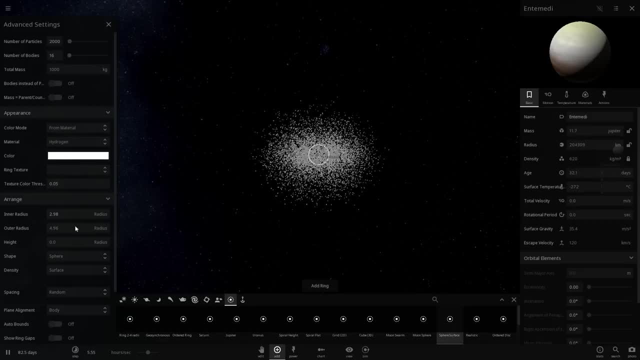 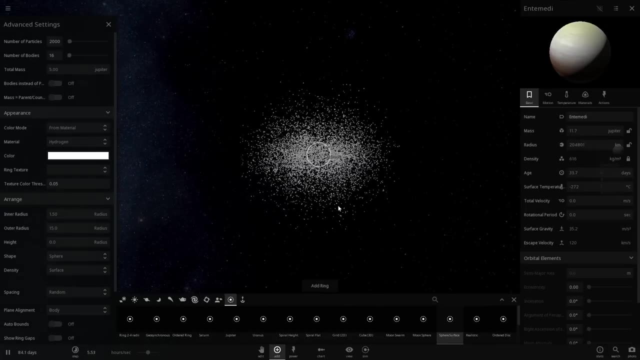 just keep adding more hydrogen here and create a larger and larger object that will eventually start becoming a star. so this is quite a lot of gas orbiting there and it's going to be a lot of gas orbiting there. and it's going to be a lot of gas orbiting there and it's going to be a lot of. 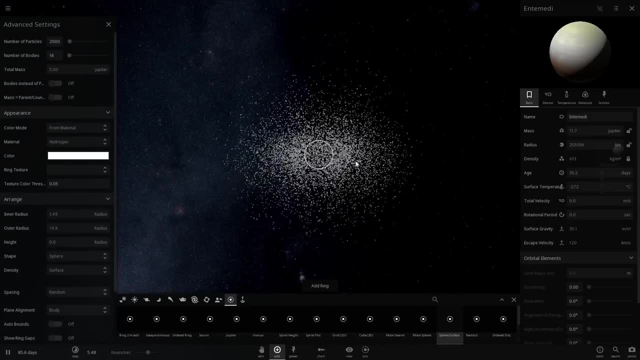 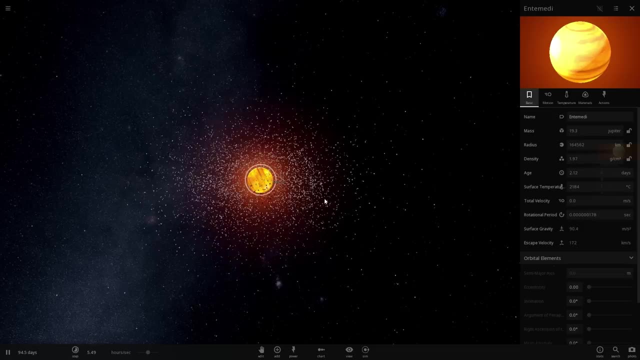 adds up to the total uh mass of this particular star and we're slowly approaching that particular situation when it's going to actually start getting really hard and becomes a protostar. so it's kind of getting closer to it. um, at this point it might actually be known as the t tori uh. 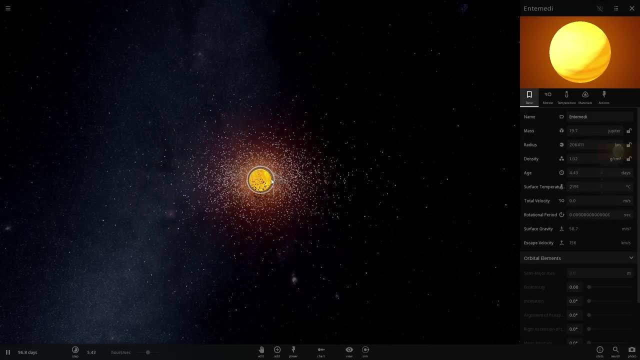 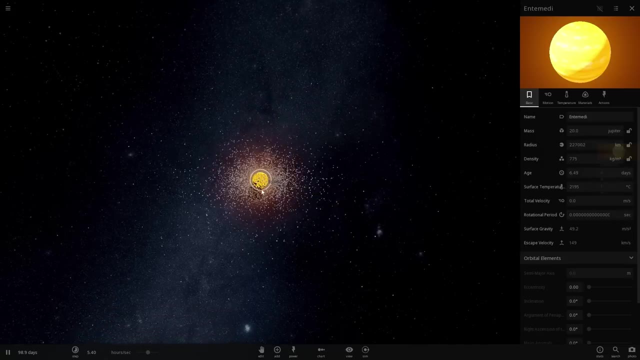 tori star, which refers to the fact that it's going to basically have um, a hydrogen burning star with really really strong stellar winds, and um usually have a kind of a really really large disk orbiting around it, which we're going to create here as well, which will eventually turn. 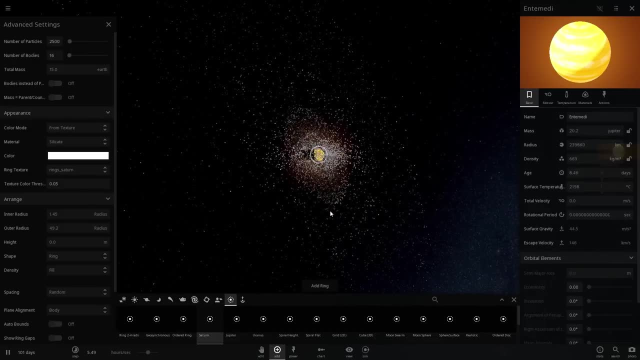 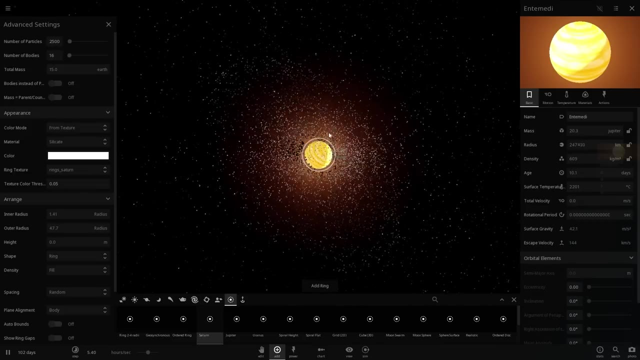 into planets, and so here is the disk that i tried to create here. it's actually spinning in a slightly different direction, but basically this disk will stay with this protostar for a very long time, even as it grows larger and larger, and eventually a lot of this material will actually get thrown. 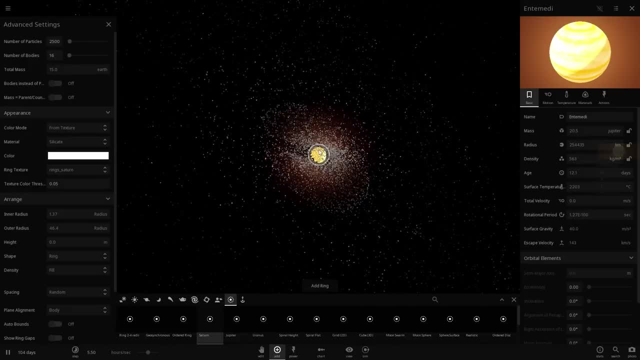 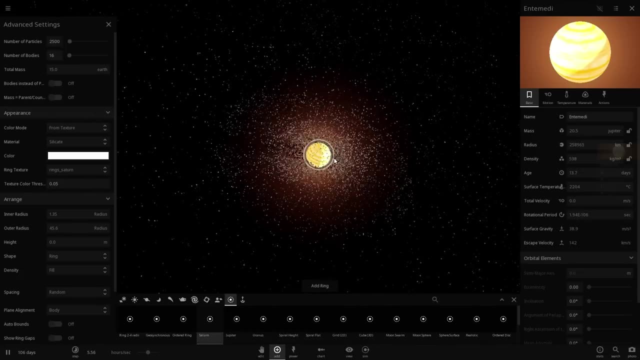 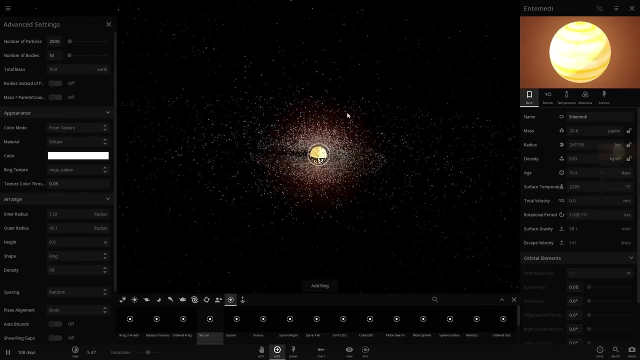 out into the outer space, because as soon as this becomes a main sequence star, basically as soon as it starts getting an actual hydrogen burning reaction on the inside and as soon as it starts getting really, really hot, the stellar winds here will actually push out a lot of this material out of the system and, as this happens, only some of the material in the ring. 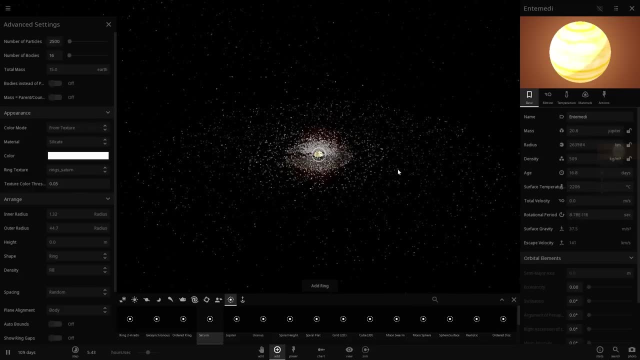 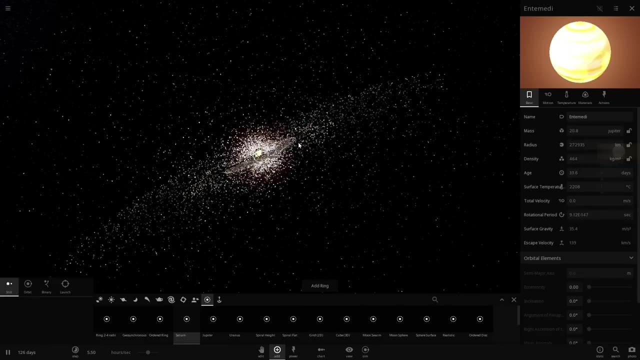 will stay and then start clumping into, essentially, planets. but before this happens, let's take a look at the actual sort of structure and, i guess, just a general look of what's actually happening here. so we have a very large, relatively hot object on the inside with a lot of stellar winds. 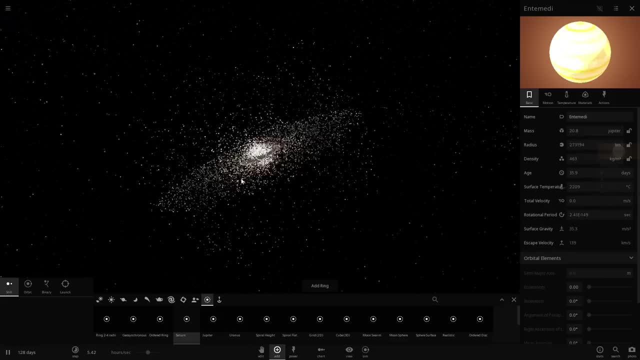 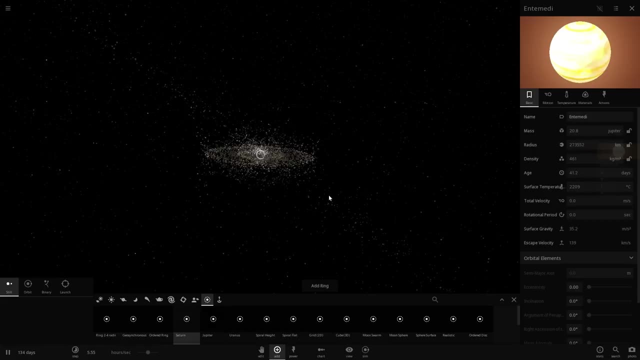 we have a lot of gas orbiting around it and we started to form this sort of ring that will turn into planets later on. but all of this is super, super thick and very, very disorganized and chaotic at first, because a lot of the stuff is just 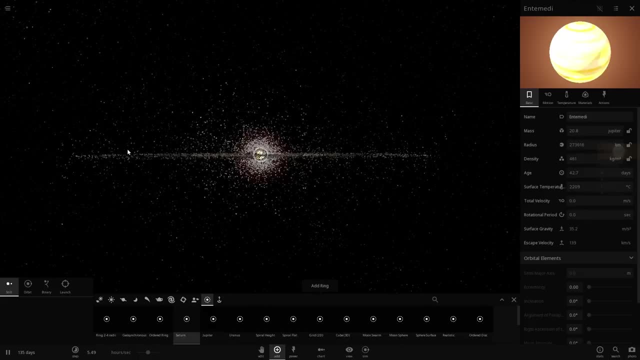 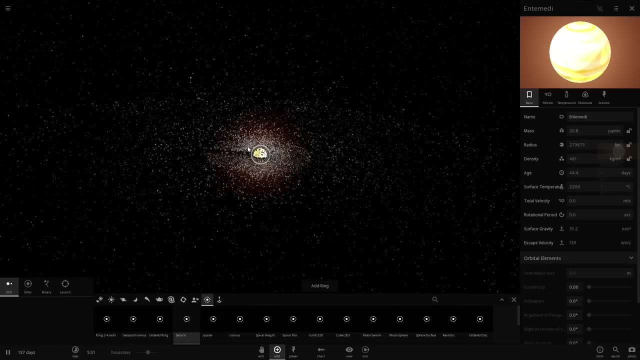 orbiting everywhere. it's not actually in the flat sort of um plane like we do have in our solar system right now. all of this is sort of all over the place and at this point, as a protostar, this particular object will actually have a lot of luminosity. it's going to be even brighter than 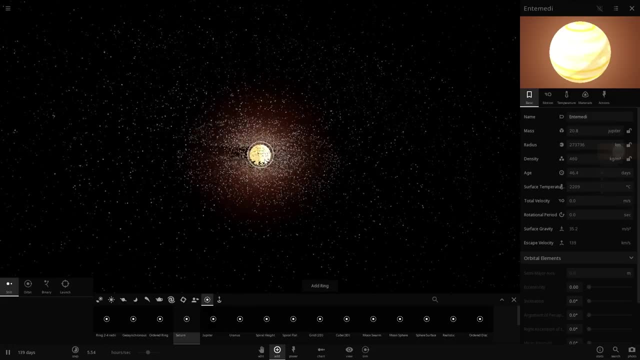 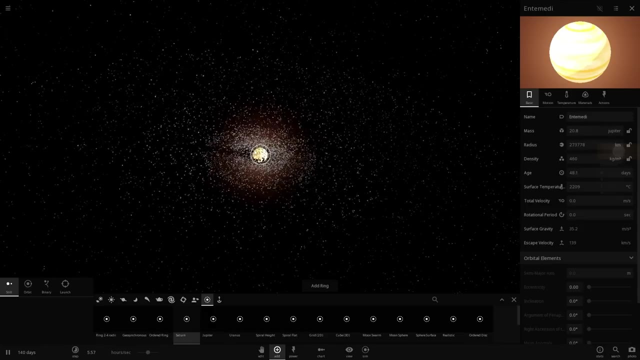 the actual star when it becomes a main sequence star size. as a matter of fact, here the size is several times larger than what it will be when it becomes a star. when it becomes a star it sort of collapses a little bit and starts burning energy and becomes 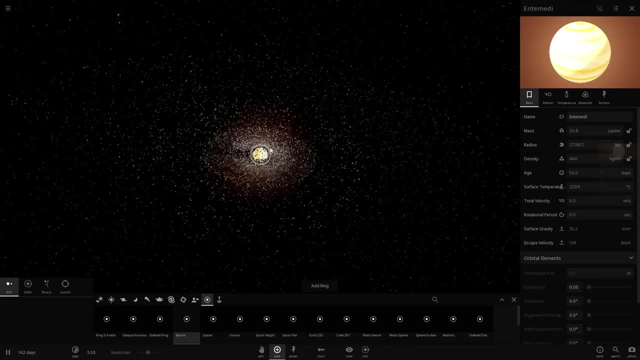 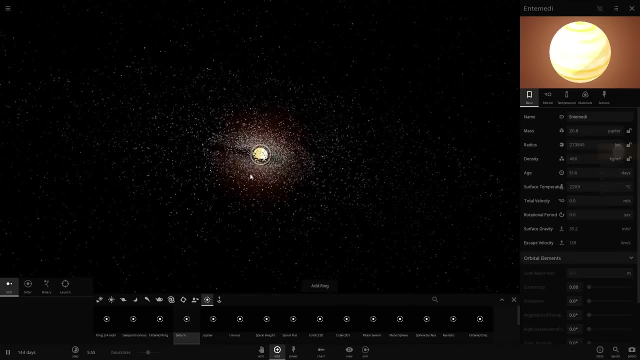 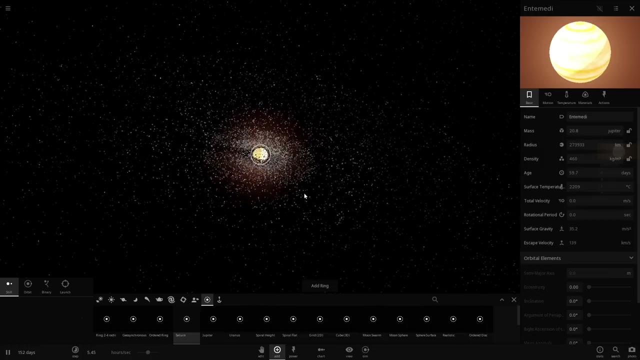 more compact, but at first, because of its essentially volume, it produces a lot more luminosity, even up to a thousand times luminosity of the actual star later on. so these objects, these protostars, are actually relatively bright and easy to see. but the thing is these objects only last. 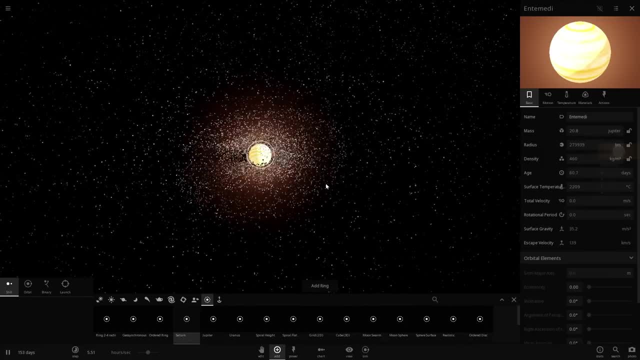 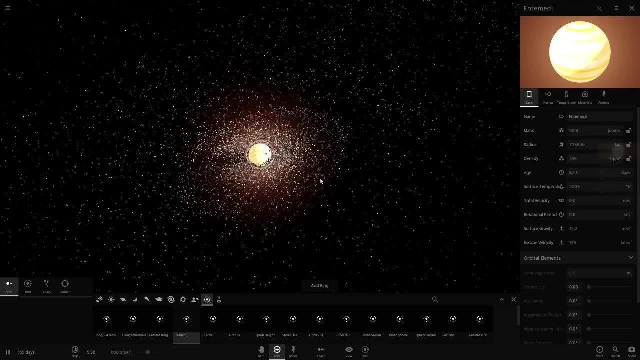 for a few million years, so they're actually quite rare in our galaxy. it's very difficult to find them, even though they're so easy to see, and generally we call these pre-main sequence stars also known as pms in astronomy, which is probably not the best acronym to use, but that's what it is, and so 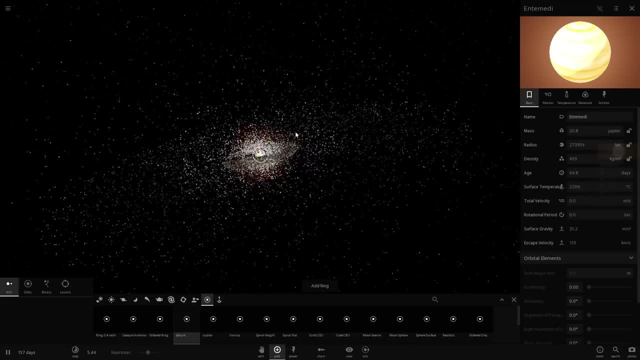 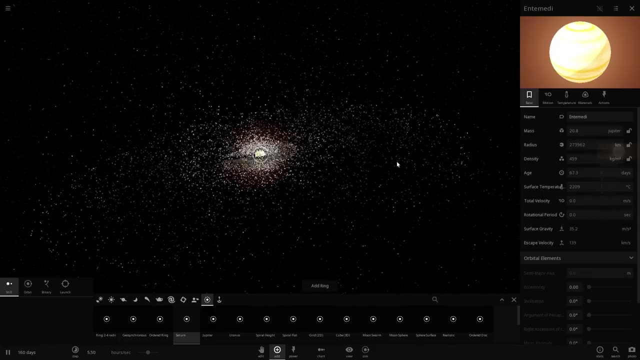 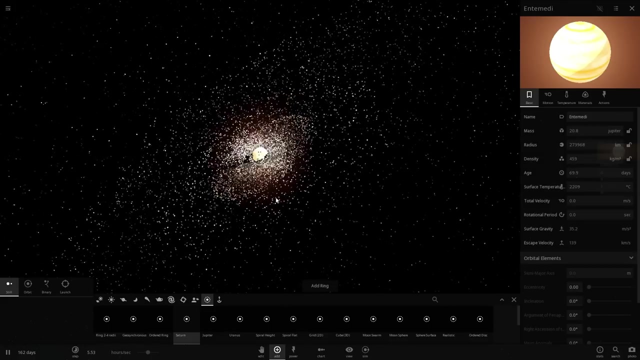 the total life of this particular object will only be several million years- usually it's about one percent of total life of the star- and these circumstellar disks- these basically disks that will later become protoplanets and also planets- also last for only several million years until all of these objects start coalescing into essentially planets. but let's just actually 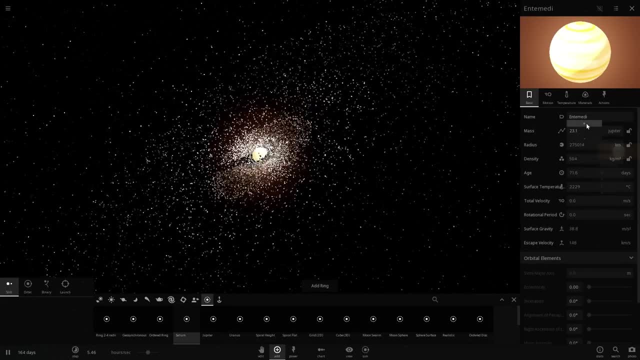 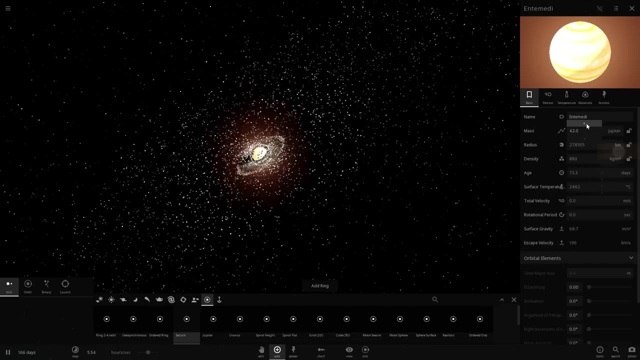 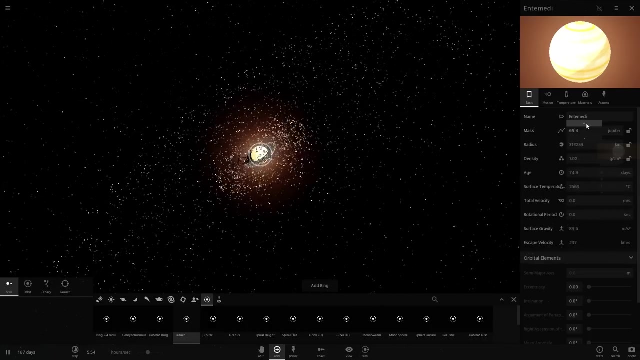 start increasing the mass here manually, just to see what this looks like later on, as this becomes closer and closer to the actual star, so all of this material will start coalescing, the actual ring will start becoming more flat and the object will eventually become a star. so somewhere around, 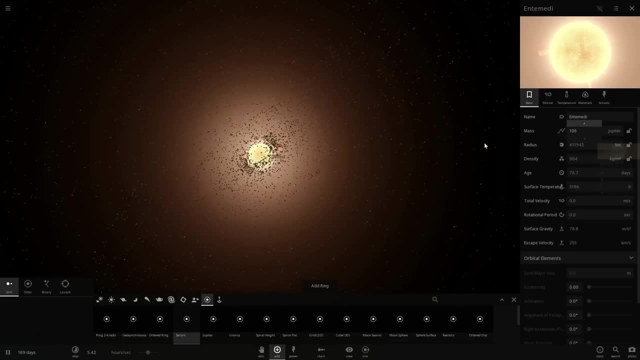 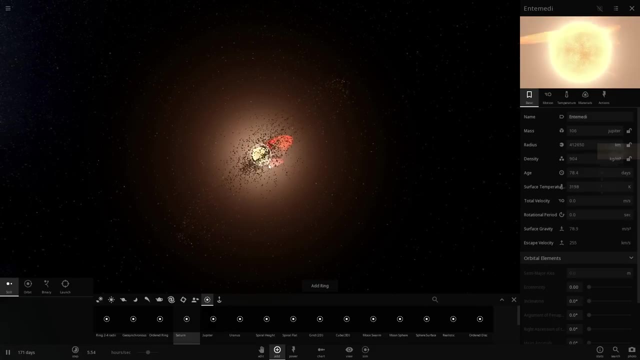 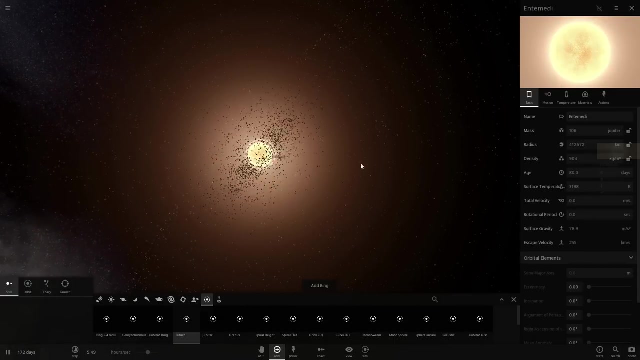 hundred masses of jupiter. this is when we'll start getting uh nuclear reaction on the inside. it becomes a main sequence star. so right now it's kind of still unstable. this is still sort of a protostar. you can see a lot of um different explosions. that's basically the representation of stellar winds. but with time this will eventually 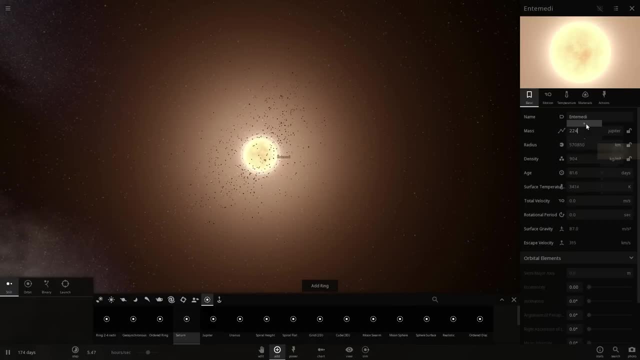 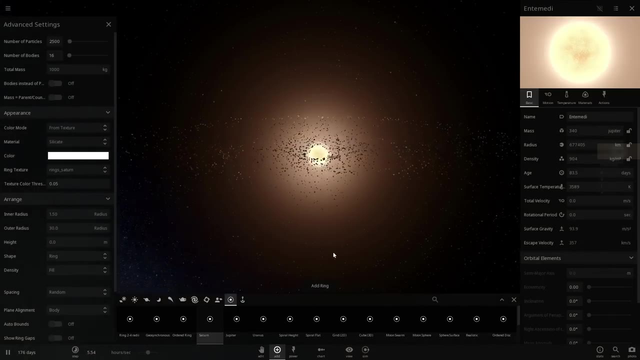 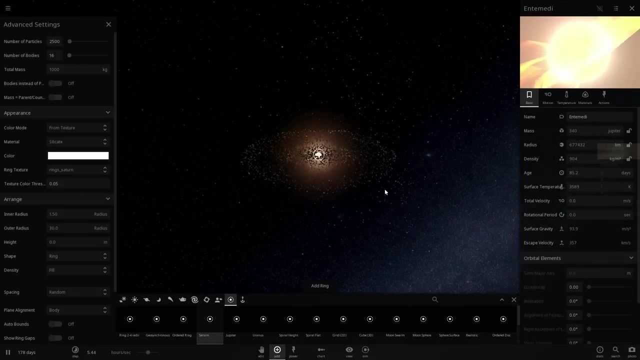 become more stable and stabilize into a main sequence star that we know as basically sun today, and the ring around it will eventually coalesce into planetary bodies which will then become planets like earth, mercury, mars and venus, and so this is essentially how the stars are born in the beginning, and don't forget that this is just one of the stars after the. 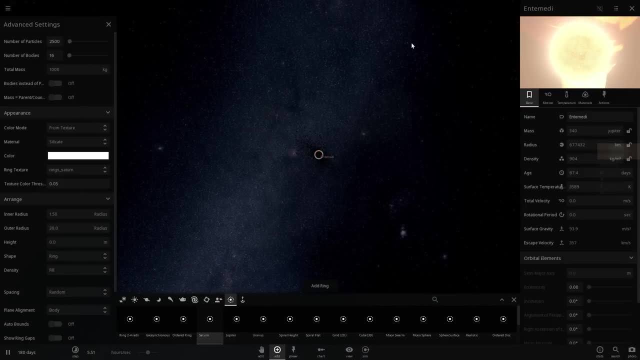 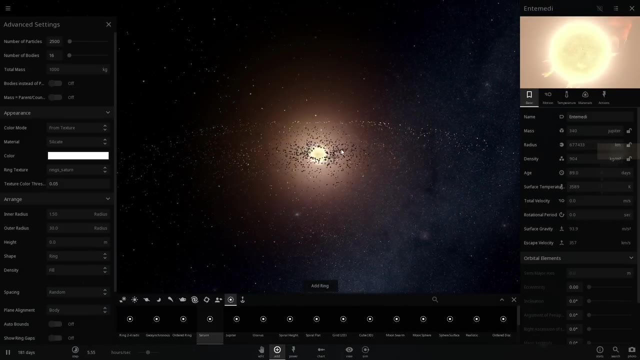 supernova, but there's going to be a lot more of them, uh, somewhere near near this region as well, and this is how, uh normally uh, star formations or star clusters are formed, and this is why so many stars, like, for example, sun and alpha centauri or proxima centauri, actually move in the same. 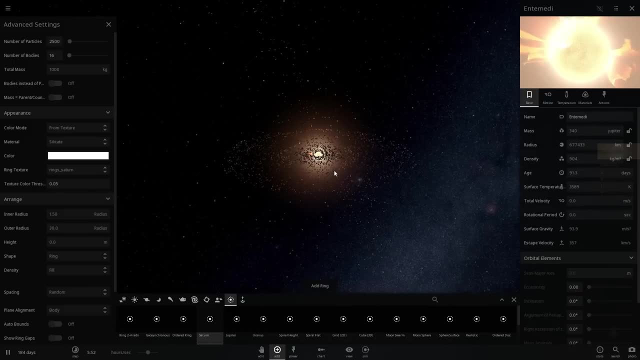 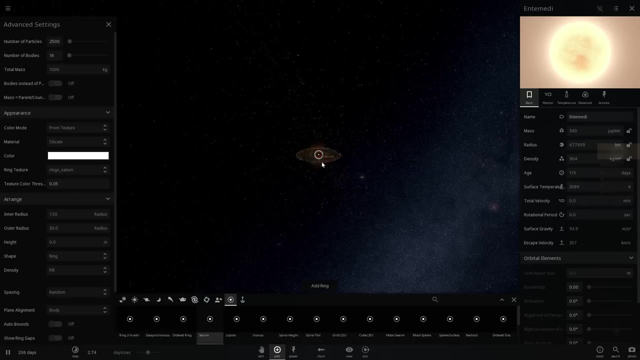 direction, because they were very likely formed in the same direction, because they were very likely for the same region from the same supernova. and if i accelerate time here, you'll see that all of this gas is still sort of attracted to the star, to the, to our intermediate star, and at some point all of 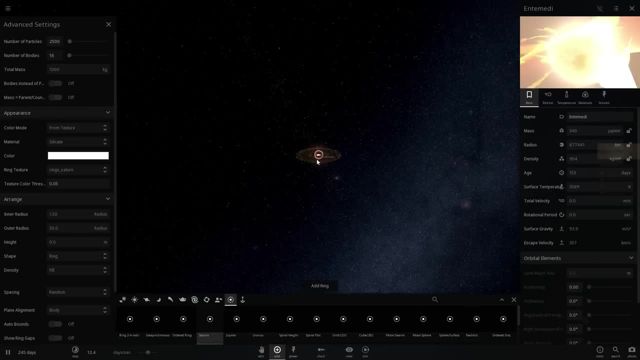 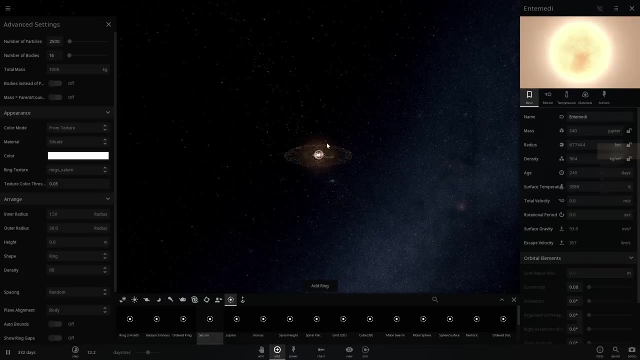 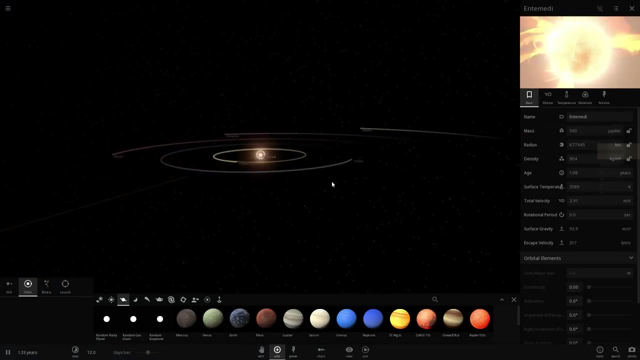 this will actually be cleared and become a very sort of a clean cut star in the middle with a protoplanetary disk orbiting around it. that will eventually, of course, turn into something that looks like this: so essentially, this will be the future of the system, when it actually becomes a.